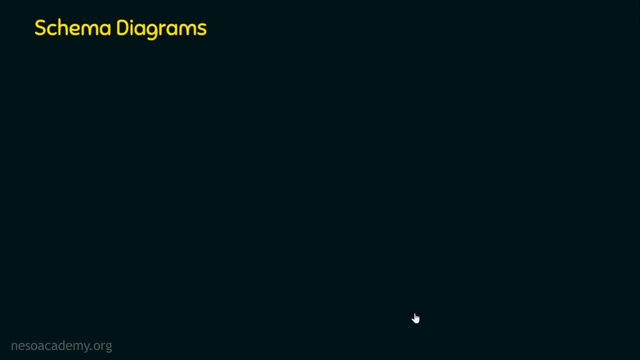 So we are now here in the topic: schema diagrams. At first let's see what is a schema. Database schema, or simply schema, is actually the logical view of the entire database. We may have a database and we want to represent the database in a logical manner, So obviously diagrams help us to convey. 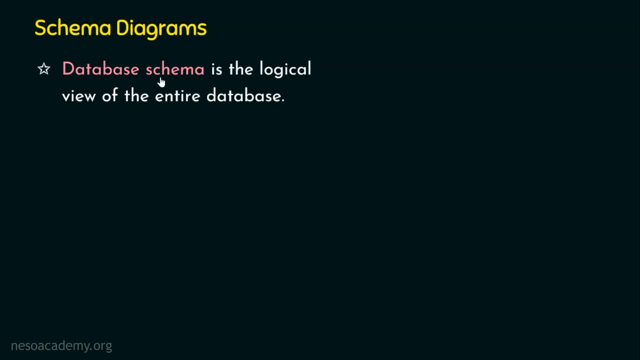 the logical structure. So schema diagrams are for the development of the database, So we can represent the database schema where these database schema is actually the logical view of the entire database And these schema diagrams are obviously going to represent the entities, like the objects. 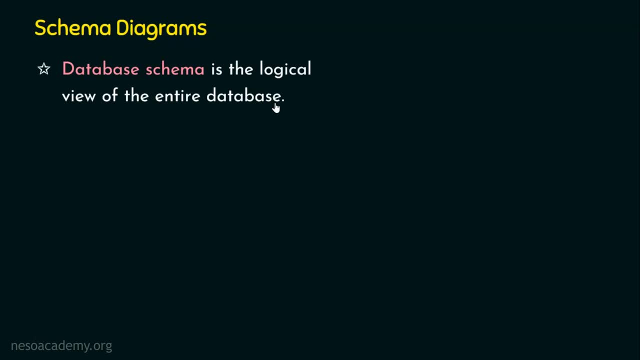 that are used. An example: object is the table name or the relation name. And if we say that there is a table, obviously this table will be comprised of attributes. So the schema diagram: it should not only display the table name as well as the attribute name, It should also focus on the 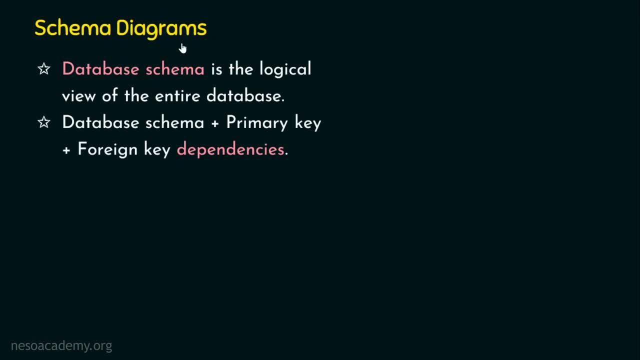 dependencies. So, in simple terms, it should not only display the table name as well as the attribute name. It should also focus on the dependencies. So, in simple terms, a schema diagram should contain the database schema plus the primary key and the foreign key. dependencies And primary key. 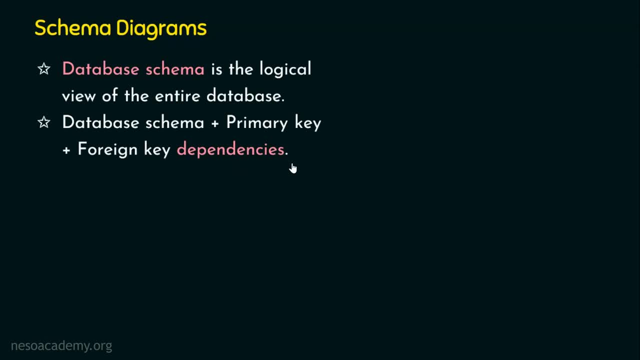 and foreign key are actually examples of constraints. I hope now we know what is a schema diagram. It is actually the database schema, along with the primary key and foreign key dependencies And how we can represent the database schema and also the primary key and the foreign key. 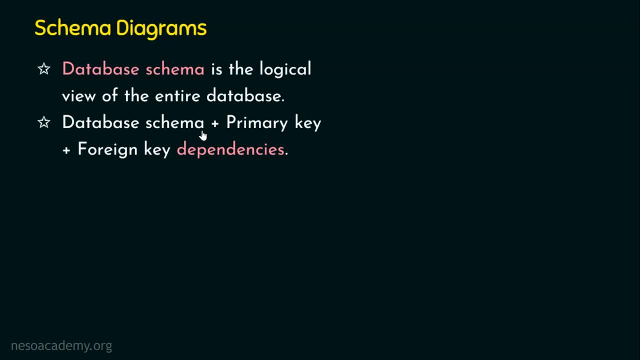 dependencies. Actually, when we talk about the database schema, and the schema will be actually having the relation name and the attribute name. So obviously schema diagrams will certainly have the relation name and the attribute name. Relation name means it's the table name. Attribute name means it's the column name. A table may have thousands. 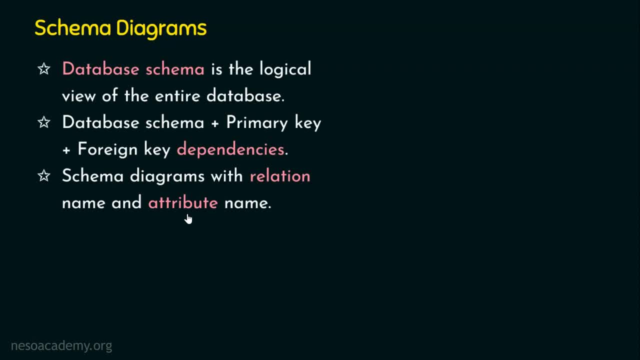 and thousands of rows. We cannot show all the data on the diagram. It's practically not possible. But we can show what is the table name and what is the attribute name. So we now understood how we can represent the schema diagram. So let's see how we can represent the schema diagram. 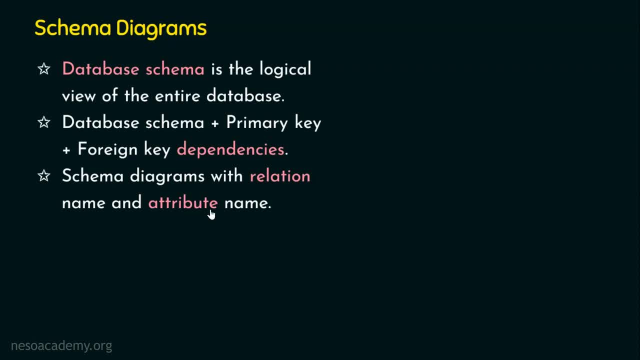 With just the relation name and the attribute name And we know not only schema diagram is going to have relation name and the attribute name. We should also focus on displaying the primary key dependency and the foreign key dependencies, How primary key and foreign key dependencies are. 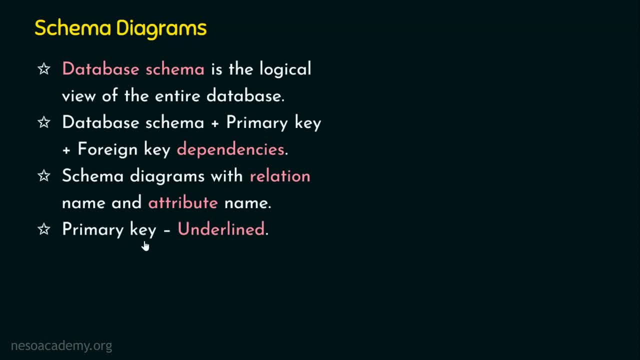 shown, Attributes that are having primary key constraint or primary key dependency are actually underlined. Then what about foreign key? Foreign keys are represented using arrows Because foreign key definitely involves two keys. So foreign keys are represented using arrows. One table is going to refer another table. In that case, which table is referring the other table? 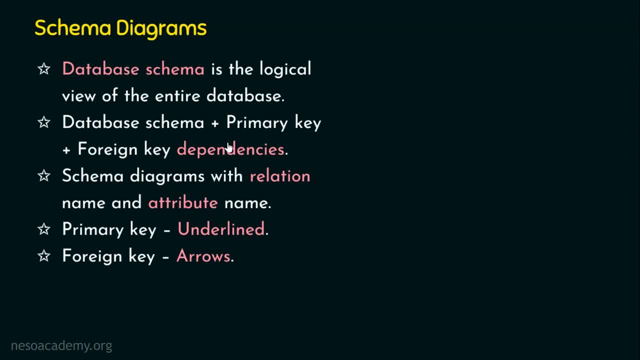 That can be easily shown using arrows. And do we have only these two constraints in reality in databases, The primary key and the foreign key? No, we have other constraints. Can we represent all other constraints in schema diagrams? No, other constraints are not explicitly shown in 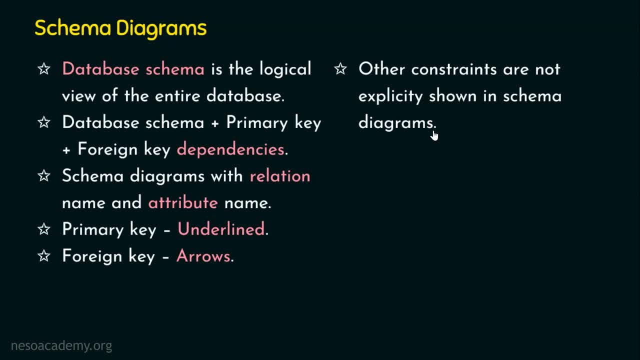 schema diagrams, And this is one of the drawbacks of having schema diagrams. Of course we can represent the logical view of the table, But we cannot represent the logical view of the table. We cannot represent the logical view of the database, along with the primary key and the 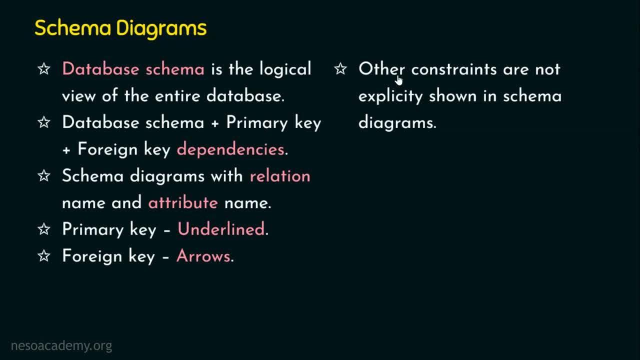 foreign key constraint dependencies, But other constraints cannot be explicitly shown in the schema diagrams. If that's the case, do we have any alternatives for the schema diagrams? Yes, of course we do have. We have the entity relationship diagrams, simply ER diagrams. 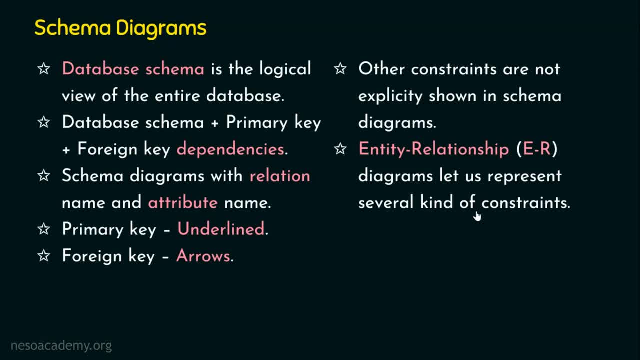 And these ER diagrams, let us represent several kinds of constraints. Like any other technologies, database technology is also seeing a lot of growth In the recent decades. So obviously many database systems provide design tools with a graphical user interface, simply a GUI interface, for creating schema diagrams. In chapter one we have seen a 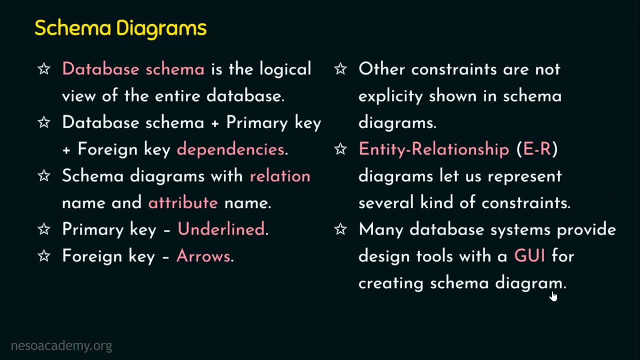 lot of database software And most of the softwares provide a design tool which is embedded with a graphical user interface in order to create schema diagrams. So whatever we have seen so far is just theoretical aspects. We need to see the schema diagram right. 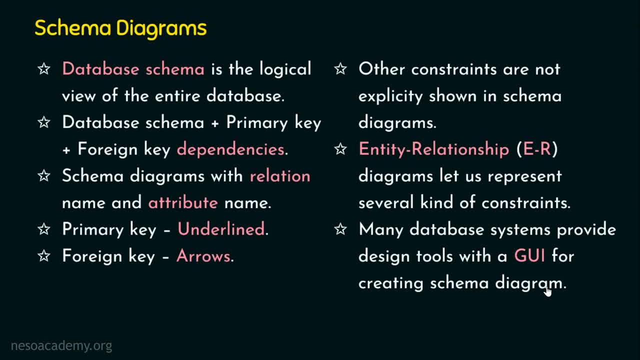 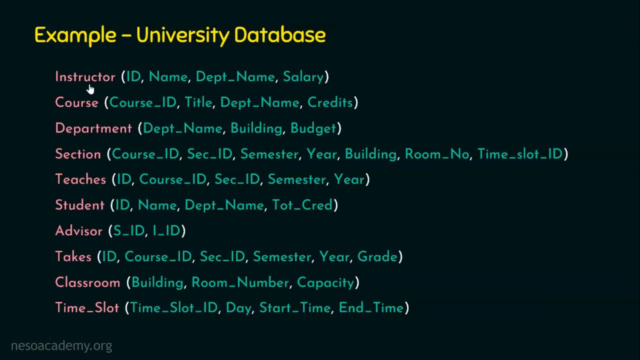 In chapter one and chapter two, which database we have taken as an example? the university database. right In this university database we have a lot of relations And we also do maintain the relationship among relations in the relation itself. Let's say how the relationship is. 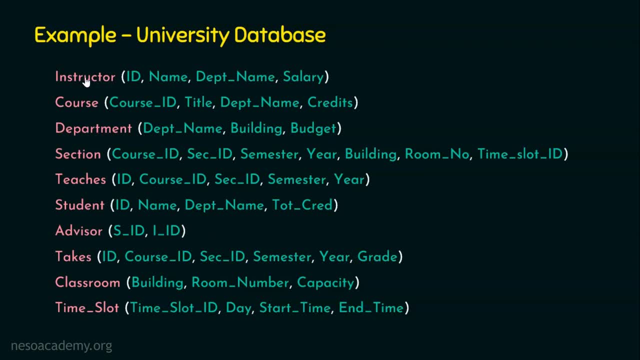 maintained. the instructor is actually belonging to a department right, So instructor will also have a department name And department relation will also have the same attribute: the department name and how an instructor and a section relation is linked. The instructor is going to teach to that particular section and this section is going to contain some. 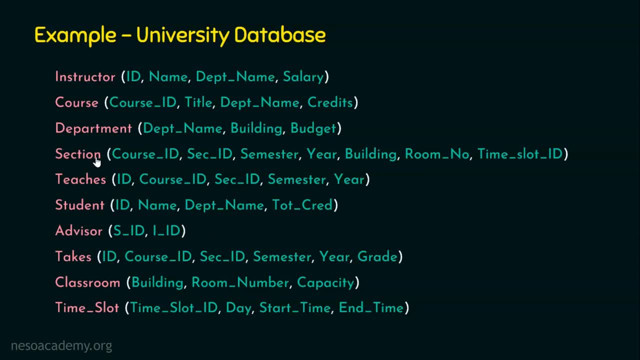 students right. So instructor is going to deal with this section, with this relationship, teaches. And what about student? Student is going to be related with this course relation. How? With the takes relationship, because student takes this course right, There will be advisor relationship. 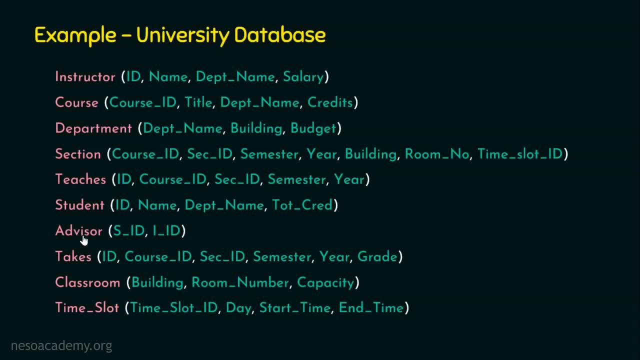 also right. So advisor is the relationship that links two tables. What are these two tables? The student, instructor table. So this advisor table will contain an attribute from the student table and an attribute from the instructor table. What attribute? The id attribute from student and the 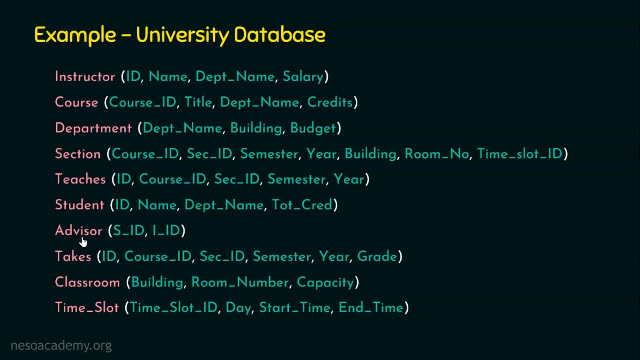 instructor table. Just pause this video for a while and just think about the relationship that are established among the relations. If the schema is represented like this, it's very vague, but schema diagrams help us to represent the logical view. Let's see the schema diagram. 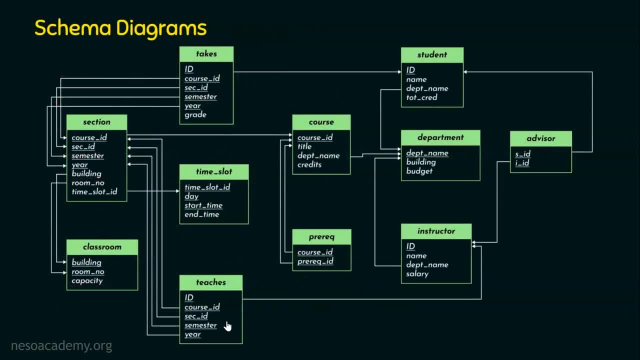 example now for the same university database. So here is the schema diagram for the same university database and if you see all the relations, whatever we have seen in the previous slide, the student relation, the course relation, the department relation, the instructor relation, 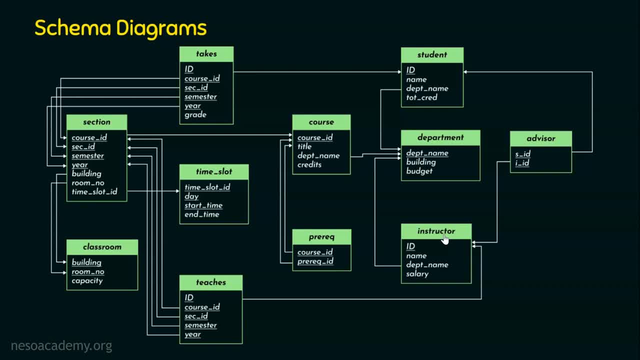 all these are relations, what we have seen in the previous slide, But how the previous slide and this slide differs. In the previous slide we represented everything as a word, but here we are representing all the relation in a diagram And what this diagram is containing Important three things. One is the relation name or the 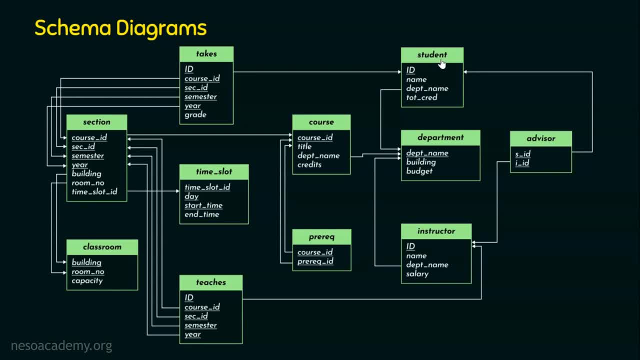 table name. In this case, the table name is student. And what are all the attributes or column names that this relation contains? The student id, the student name, the department name and the total credits earned by the student. Let's take the same student table, The student id or. 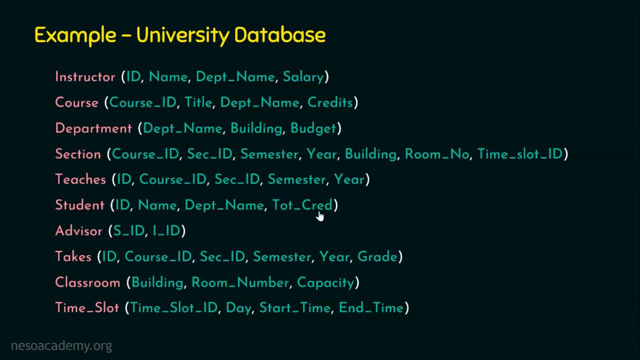 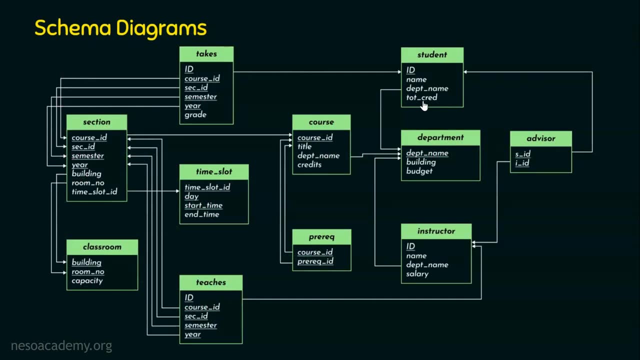 simply id name, department name and total credits. Four attributes. The same is represented here: Name and total credits. And can you see one of the attributes is different from other attributes? Yes, id is underlined. What do we mean by this? It means this is a primary key attribute and that's. 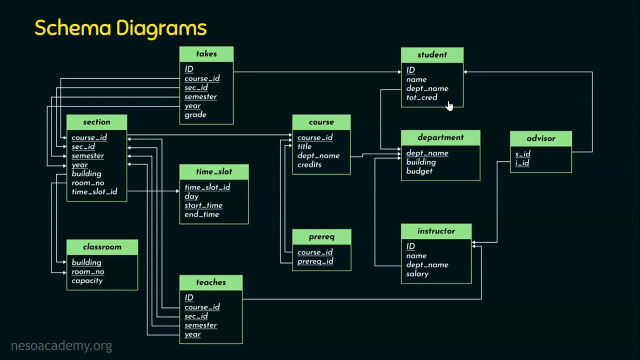 why I told you the primary key attributes are shown with an underline. So here id is underlined. So obviously id attribute is a primary key attribute. Just pause this video for a while and think about the other primary key attributes in the schema diagram. I hope you are done So. 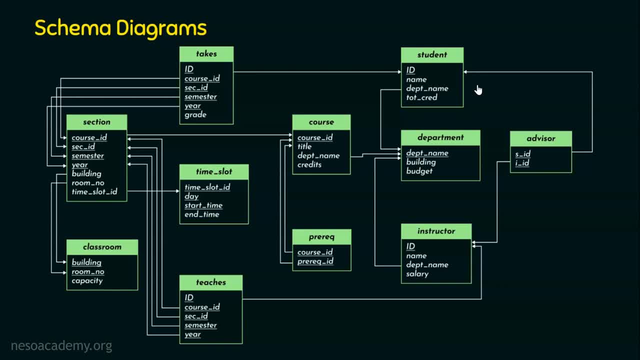 whatever is underlined, all these are primary key attributes. And, coming to the arrow, can you see here This is student relation and this is instructor relation And this instructor relation also has id name, department name and salary. So these four information or four, 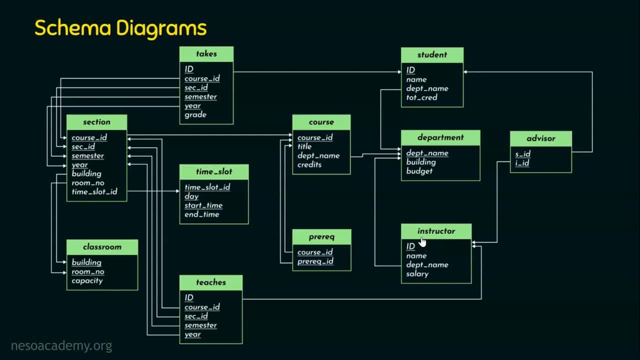 attributes are belonging to the relation instructor, How this instructor relation and student relation are linked. Every student is assigned to an instructor with the advisor relationship. I have already explained this in the previous lectures. So student and instructor are related with this advisor relationship. And what are all the two? 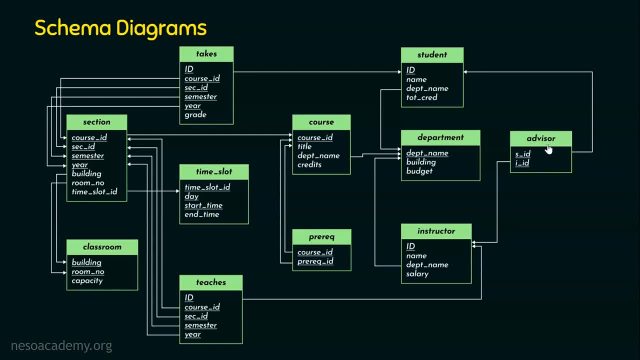 important attributes this advisor relationship should contain. It should contain this id that I am representing it as student id. But why I am representing as student id is that if I simply take id here and if I simply take id here, this relation has two column names with the same name. 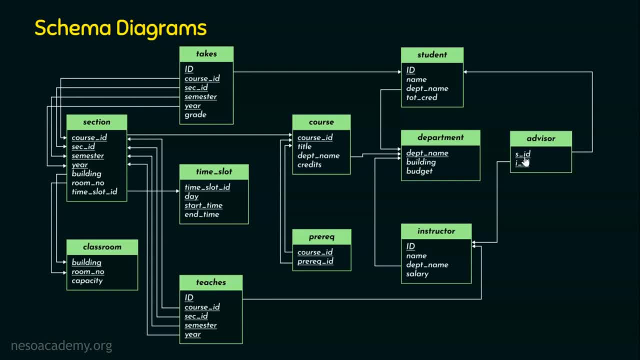 id id, But we don't know what id it is, whether it is a student id or instructor id. So I am representing it as s id, which means this is student id, which is this id, And also i id represent that it is instructor id, which is this id. So this is how relationship are. 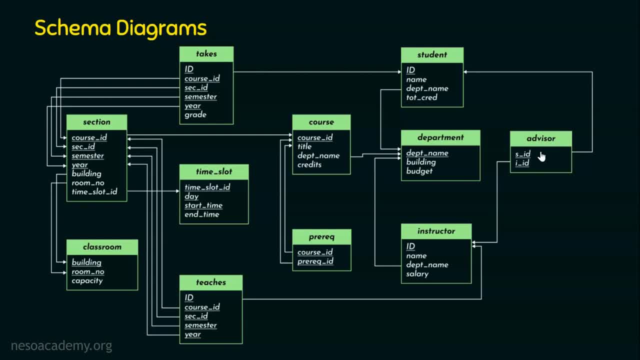 maintained. Let's see how the instructor and section relationship are maintained. Here is the instructor relation And where is the section relation. Here is the section relation And how the instructor and section relation are linked. An instructor will be teaching to that particular section, right, So instructor. 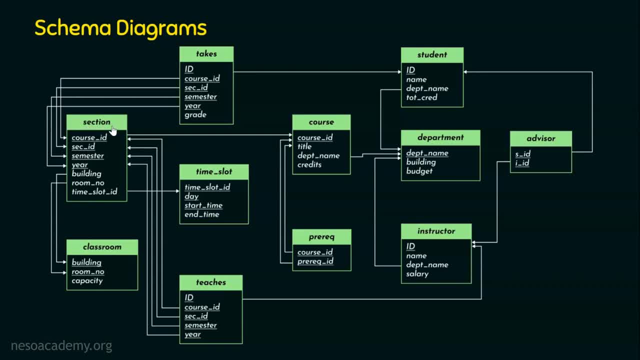 this particular section And this section will be in a classroom, right. So this section is having a classroom And this classroom will be in a particular building. the room number and the capacity of that particular classroom And student takes course, right. So where is the student? 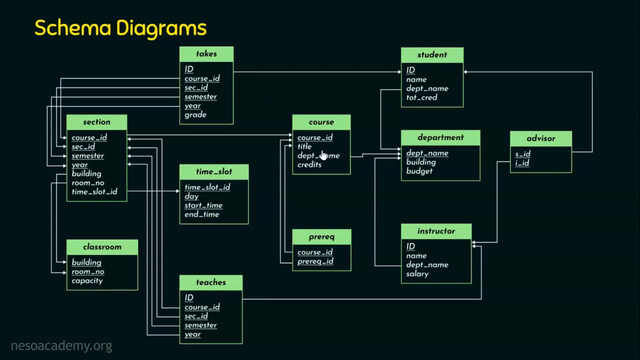 relation Here. So here is the student relation, Here is the course relation And student takes this course. Can you see here This takes relationship, is there with the student. We have seen underlined represent actually the primary key And can you see the foreign key constraint? Just see this example. 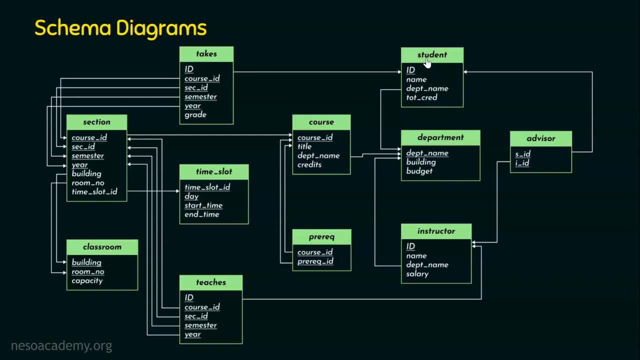 the student relation and the department relation. In the student relation we have an attribute called department name And in the department relation we have an attribute called department name. And this is the foreign table, And this foreign table contains department name as the. 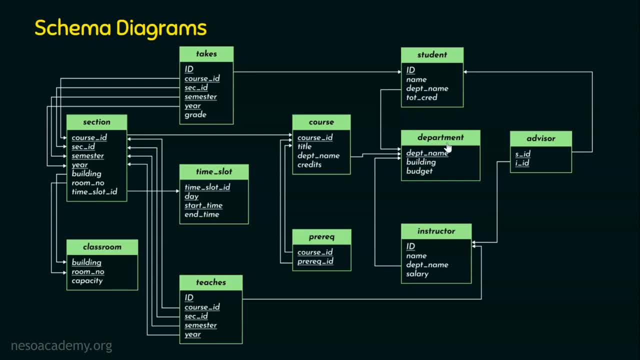 primary key attribute And this primary key attribute in the department table is actually linked to the student table And this student table. here it is not a primary key attribute because in the student relation there may be multiple students belonging to the same department, Whereas in the department table we need to have the department entry only once. 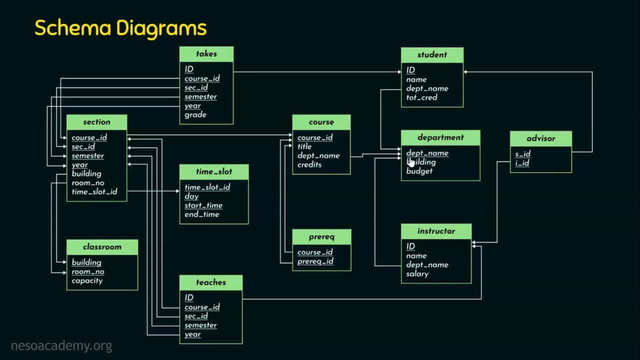 And that is why this department name in the department table is having only one entry And that is why this department name is a primary key attribute here And the foreign key representation here is: the student table is referring to which table? The department table. That's why the arrow is like this: Can you see: student table is referring the. 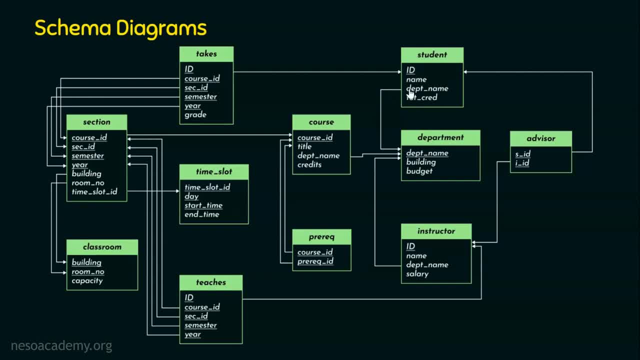 department table. So whenever any entry is made in the student relation, the department name will be validated or the referential integrity is validated by referring to this table. Suppose, if we are entering a department name here, this department name should exist in this table. So 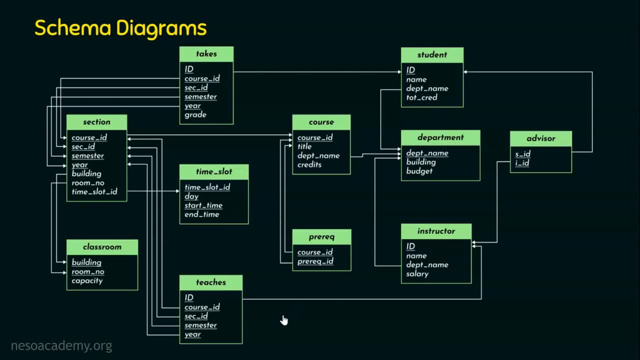 I hope now you understood the significance of having schema diagrams in databases. And that's for the day. In this presentation we have focused on the schema diagrams and the significance of having schema diagrams, But the drawback of this presentation is that we are not going to be 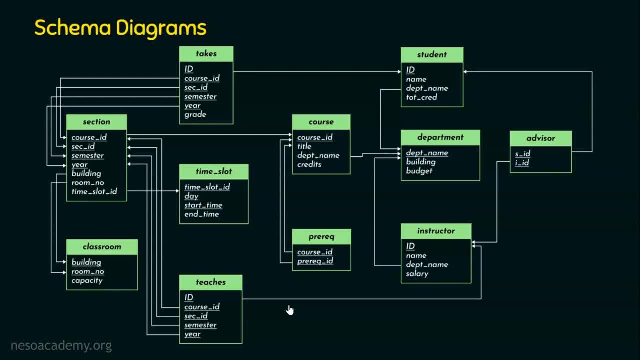 able to represent other constraints, And the drawback is in this schema diagram we can represent the relation name, the attribute name, along with the primary key and foreign key constraints. Can you see here only primary key- the underline- and the foreign key- the arrows. 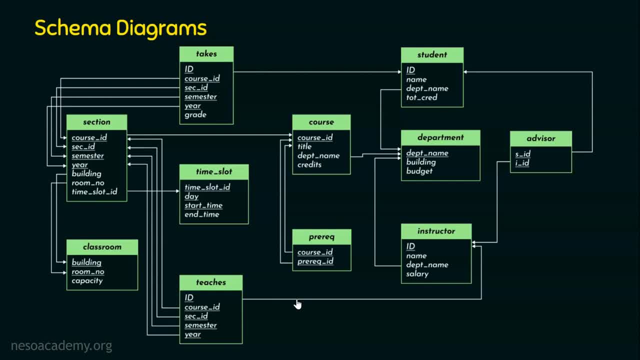 can be represented And we are not able to represent other constraints. And this drawback is overcome in which diagram? The entity relationship diagram, the ER diagram. We are going to focus on ER diagrams in the next chapter And I have not explained the relationship between. 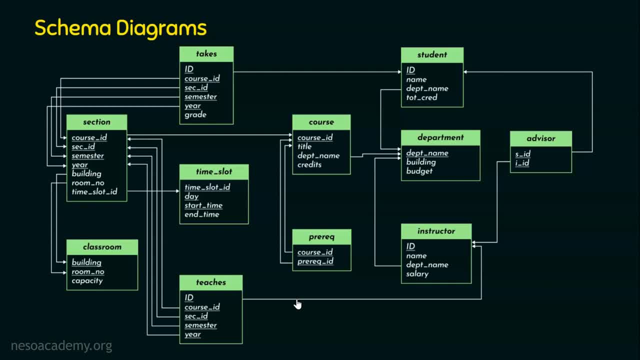 the section relation and the course relation and the relationship between the course relation and the prerequisite relation. This is the homework for you. Just pause this video for a while and just think how the relationship is established in the entire schema diagram. I hope the session. 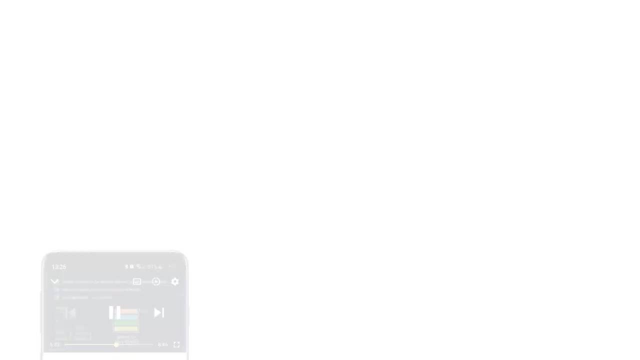 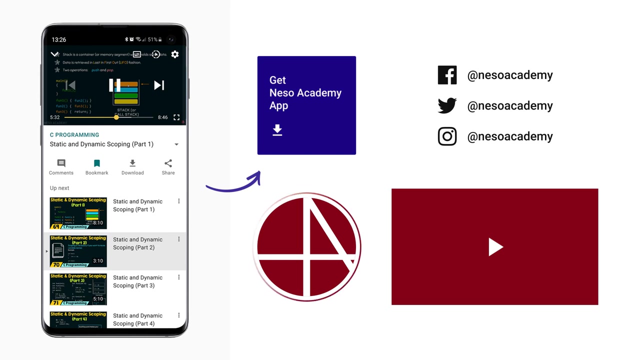 is informative and thank you for watching. Thank you.